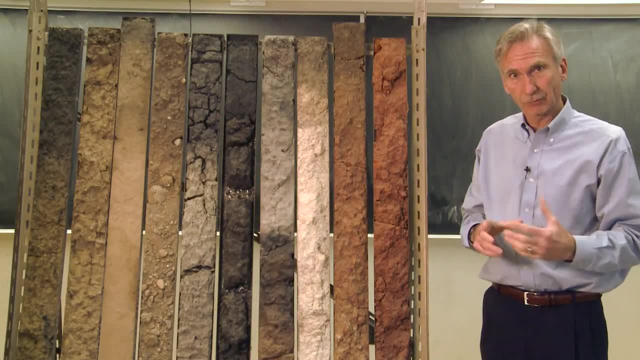 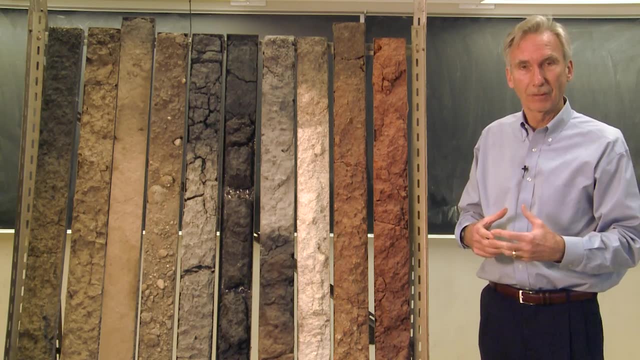 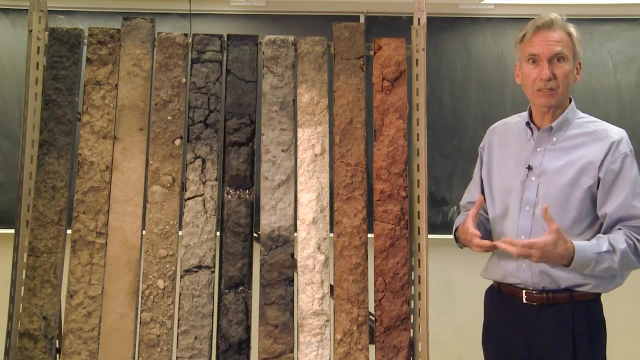 have black colors, So we have this wide range of different colors, And we can use colors to actually help us define soil horizons, And so what I'm going to do over the next couple of minutes is define for you the soil horizons, the six master horizons that we can find in the soil. So I'm going to start. 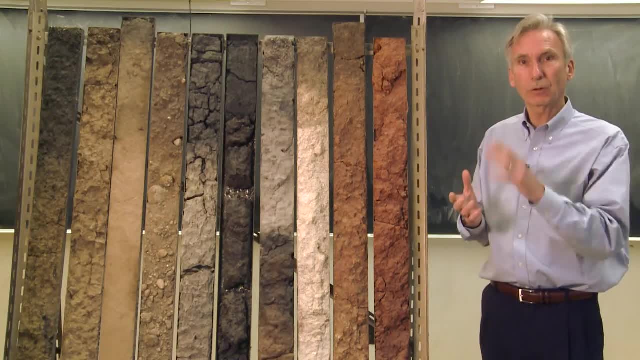 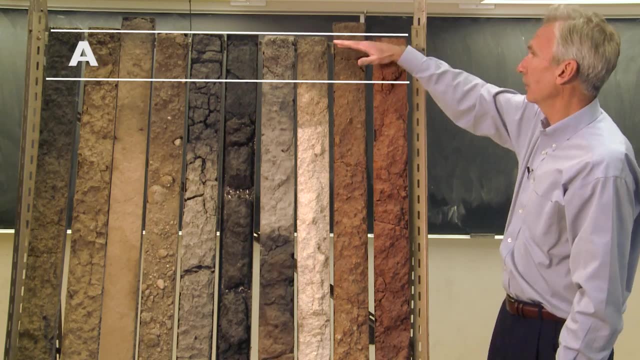 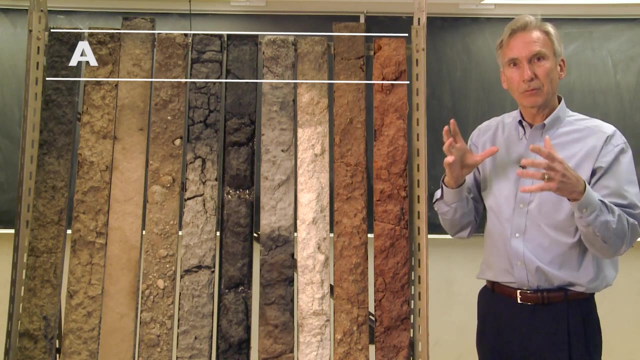 off talking about the topsoil. The topsoil is the A horizon And the A horizon is at the very top. It's usually dominated by organic matter, as you can see in these profiles. So organic matter imparts a very dark color, either black or dark brown. That is typically. 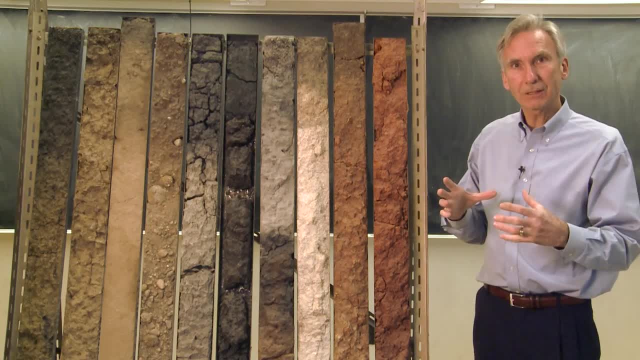 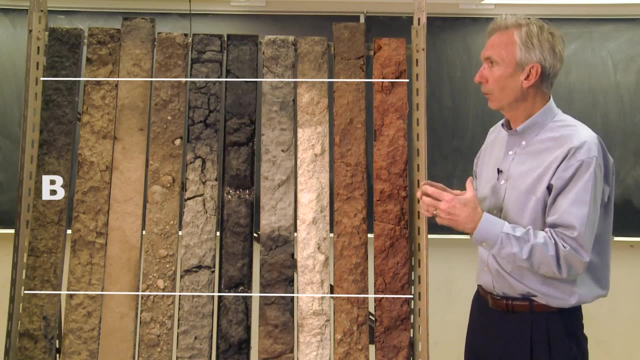 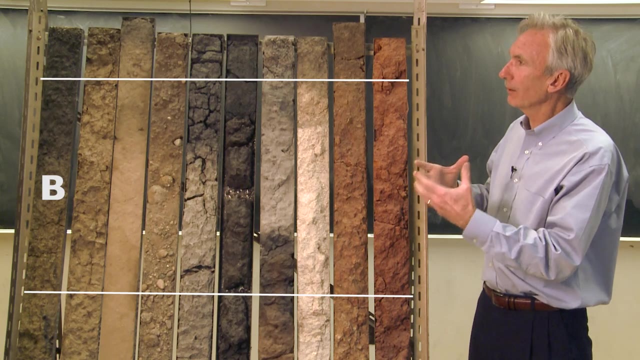 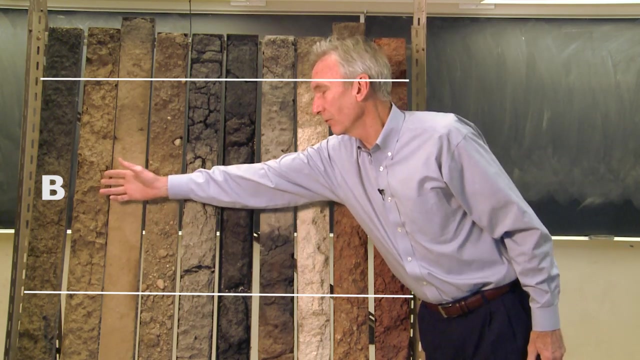 the soil of an A horizon. A B horizon is called the subsoil, And the subsoil is where everything has accumulated, So as soils, weather. what happens is that things sort of move out of the A horizon and they accumulate down in the B horizon. So over here we have nice. 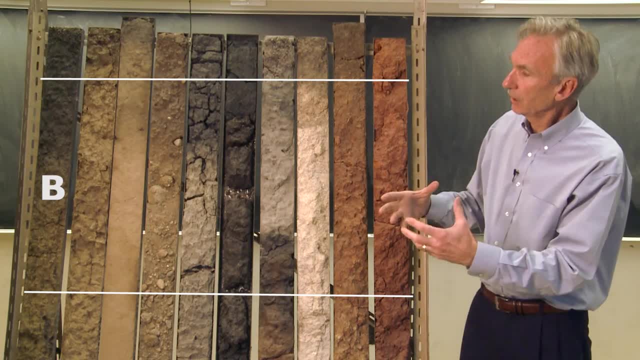 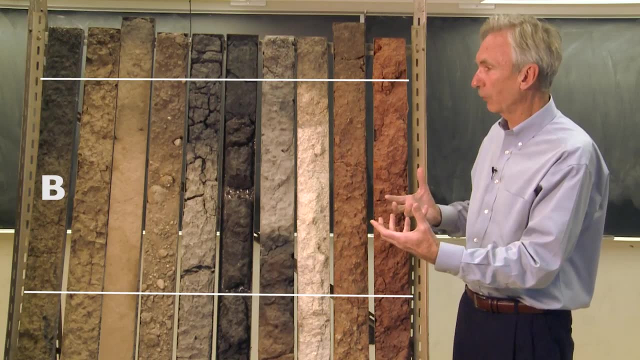 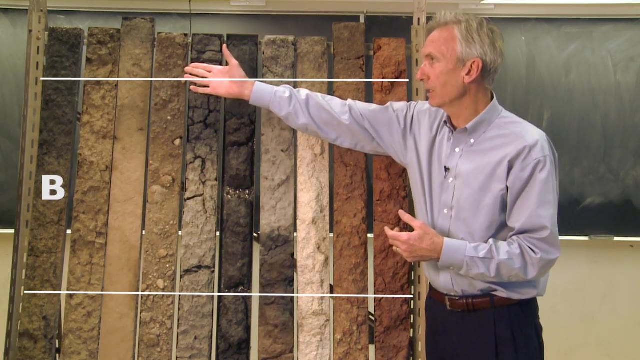 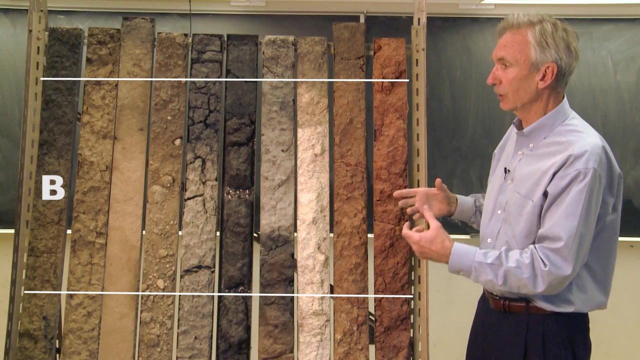 B horizons. A B horizon has a higher clay content, So, for example, it would be like a silty clay loam texture in the B horizon compared to the top horizon, which would be probably a silt loam. So the B horizon is the horizon of accumulation. It is also the horizon which 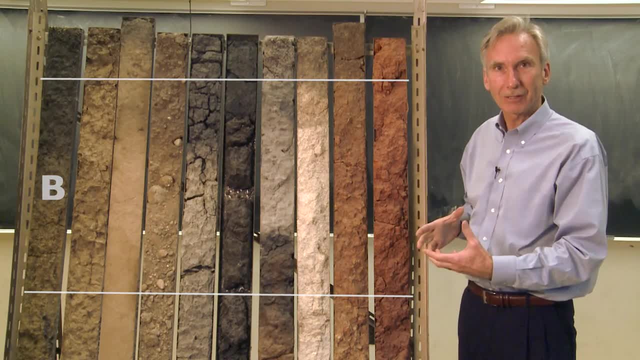 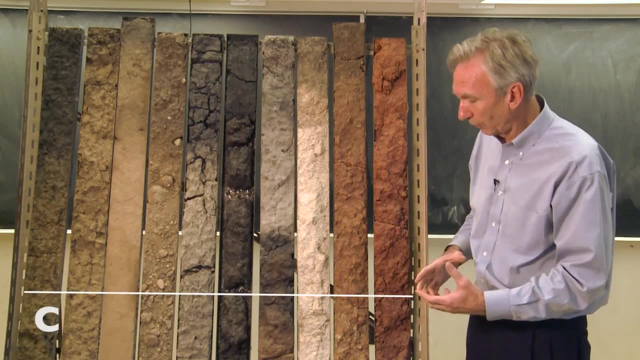 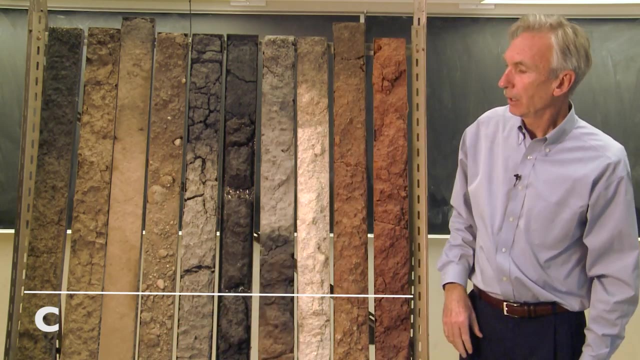 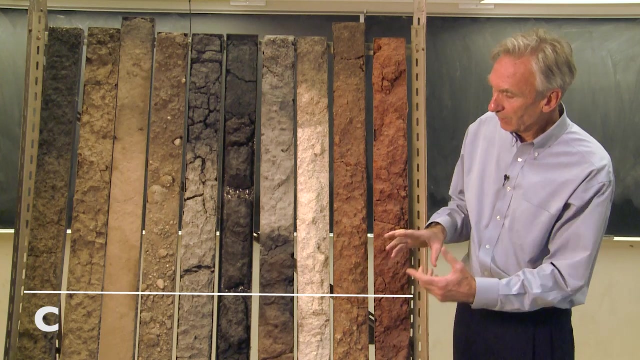 is most colorful in a soil is the B horizon. The C horizon is the parent material And that's the material from which the soil formed. So at the bottom of this profile here and that profile and the profile on the far left-hand side, those soils over there, all right, which you're actually looking at, is called the. 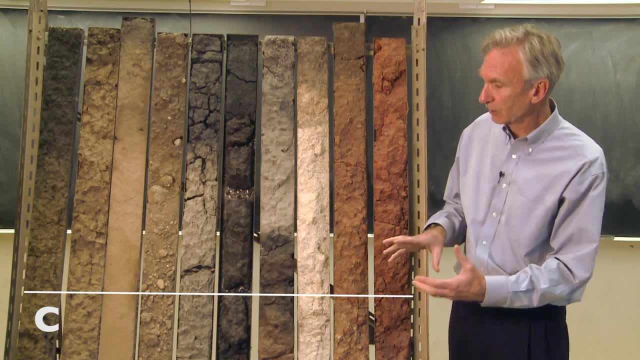 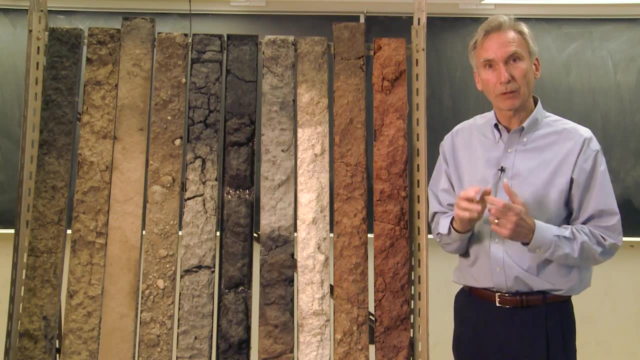 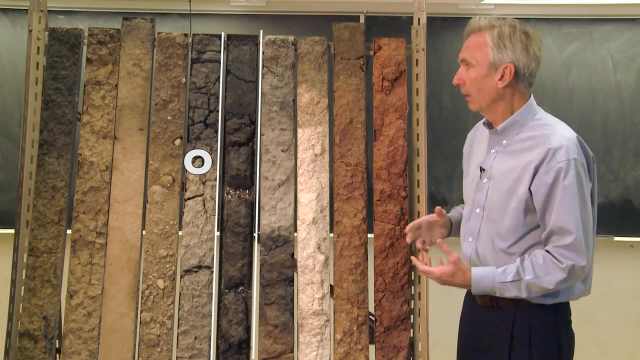 parent material And again, that's the material from which the soil was formed. So those are three of the master horizons. We have three others that we use. One of them is called the subsoil, The other one is called the O, And the O horizon stands for organic, Usually the O horizon.